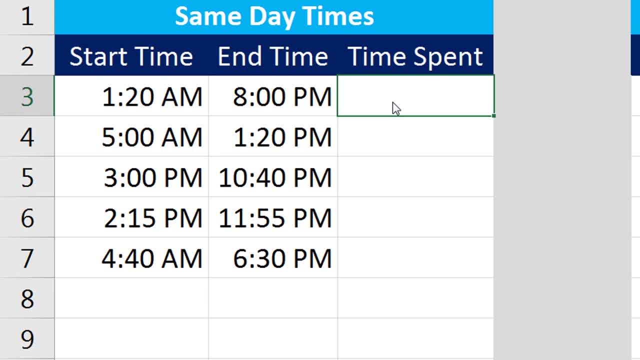 I will remove the start time from the end time, Since the end time is a larger value compared to the start time. so what i would do is i'll simply press equal to on my keyboard while i have this cell selected under time spent, and then i will select the greater value first. 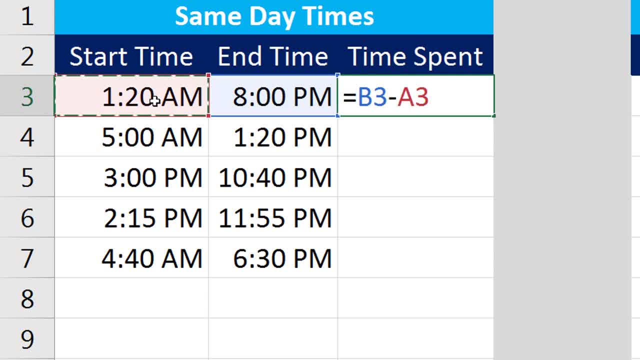 minus the smaller value, that is the start time, and then i press enter on my keyboard. i have the time spent, but it is showing me the value in a am or pm kind of format and i don't need that. i need proper number of hours instead of having pm tailed with that one. so what i would 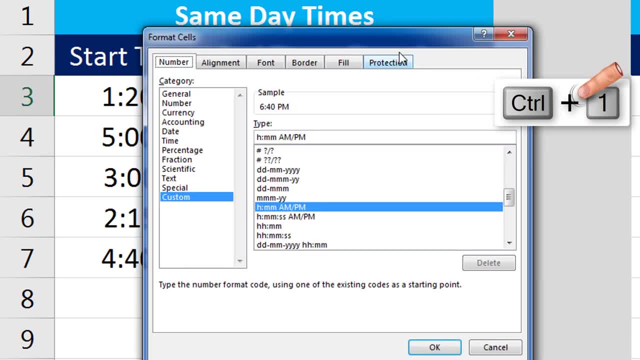 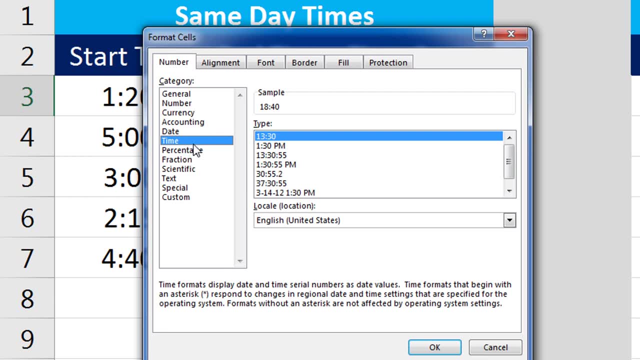 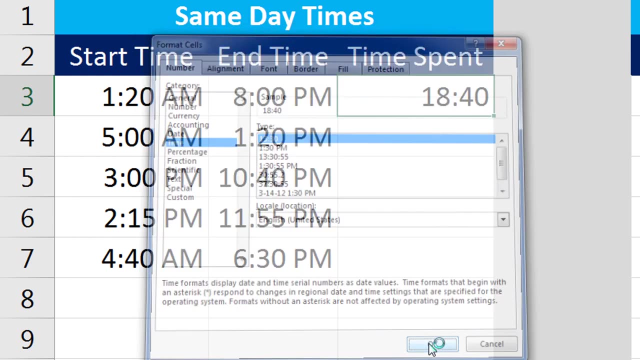 do is i will press ctrl 1 on my keyboard to bring in the format cells window. under this dialog, i can simply select time from the category column and here, under type, i will select 13- 30. that is the number of hours i can now see. i have 18 hours, 40 minutes spent. 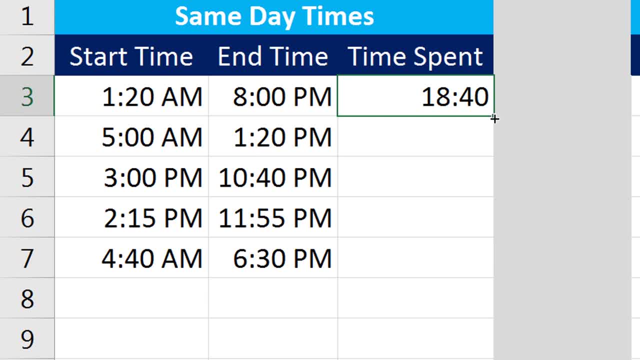 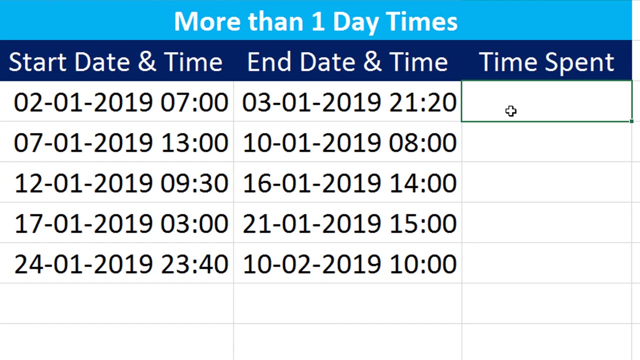 on that day. if i drag this down, i have other values properly calculated in a similar format. now this is how we calculate the difference of times between any given time of the same day. now let us take a look at calculation of times if we have more than one day. so we have this data set. 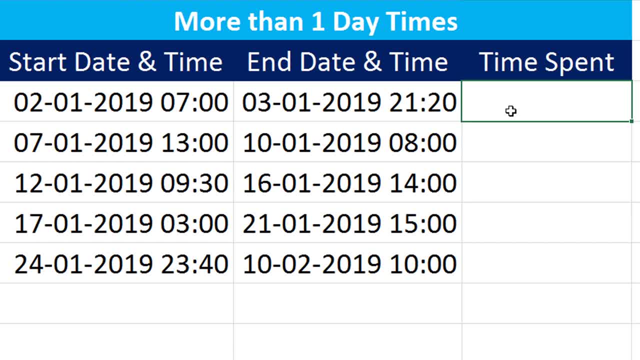 that is showing us start date and time and end date and time with different days. so what i would do is i will remove the smaller one from the larger one, so end date is a larger one, start date is a smaller one, remember that, so i will press. 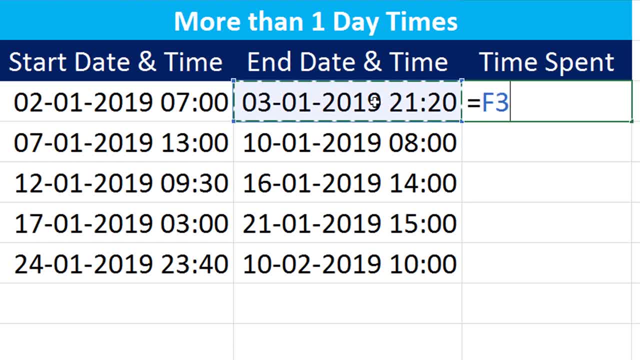 equal to on my keyboard, select end date minus start date, and then i press enter on my keyboard. i get the time spent, but in a different format. i don't need this. i i need a friendly format like how many hours and minutes have been spent on the same day. so i will press ctrl 1 on my keyboard and then i